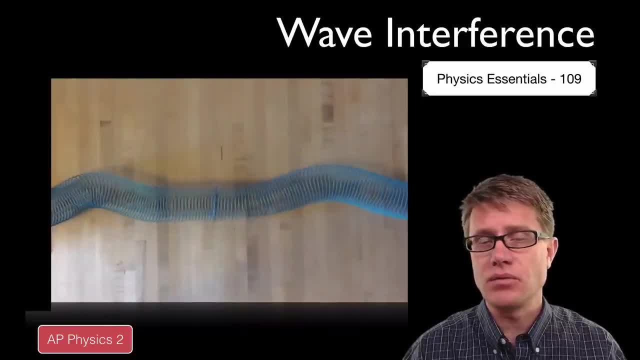 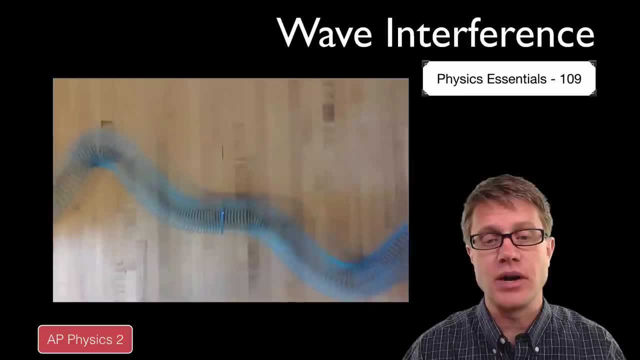 on the same side. We do not know if they bounced back or if they went through, So a better way to figure this out is to send waves on either side. So I am going to send a wave from the left on the top and from the right on the bottom. You can see they interact. But now the wave. 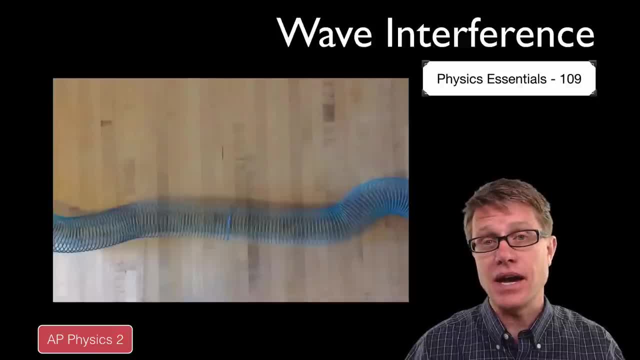 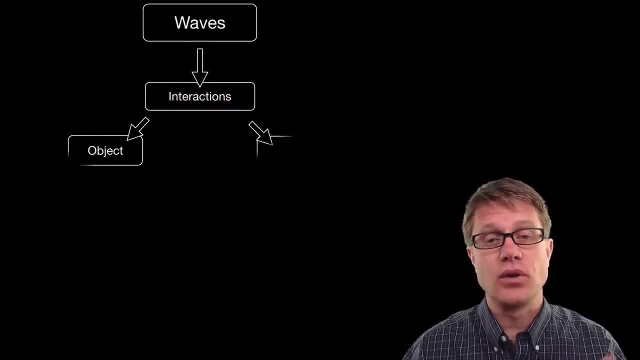 on the bottom continues to the left, And so when waves hit, they interact, but they move through each other. They are not reflected off of each other, And so wave interactions can take place when a wave interacts with an object, hits an object or hits another. 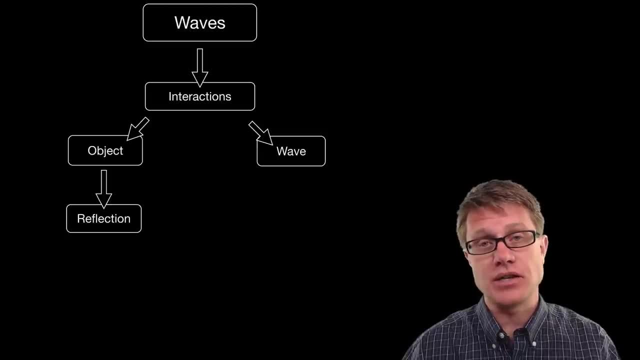 wave. So when that interaction is with another object, we get reflection. It bounces back. Now it depends on what we are hitting. So if it is a fixed object, the wave- for example the slinky- hits something that does not move- it will actually be inverted when it comes back. In other words, the wave goes. 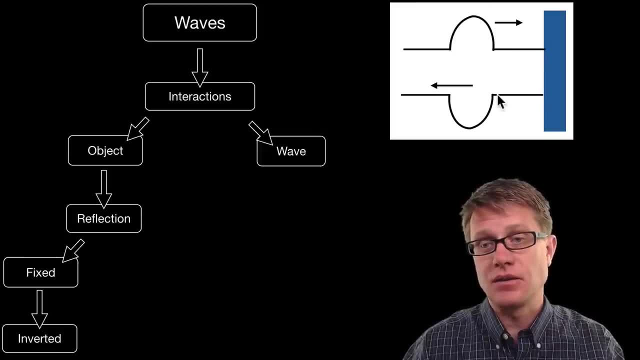 in this direction: It is on the top, And when it comes back it is going to be on the bottom. That is only if it is a fixed object. What happens if it is a free object? Well, the opposite happens, And so, as it comes in now, let's say that this is able to move back and forth. 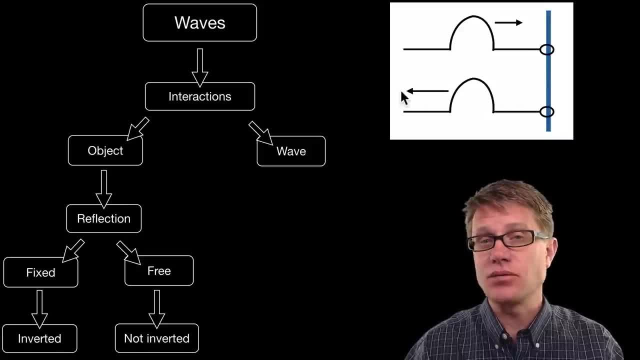 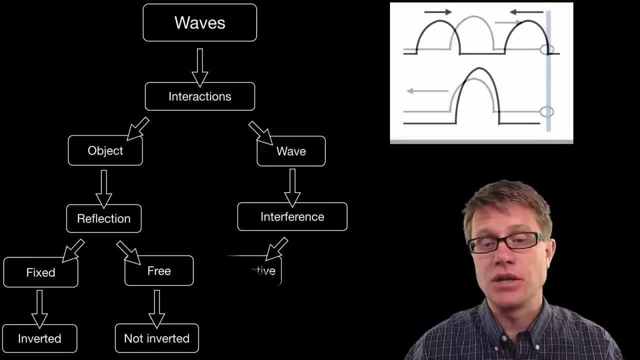 the wave comes in on the top and it goes back on the top And so that is reflected. So we get reflection. Now, when waves hit each other, we get what is called interference, Two waves interacting. That interference can either be constructive. Constructive is when two waves 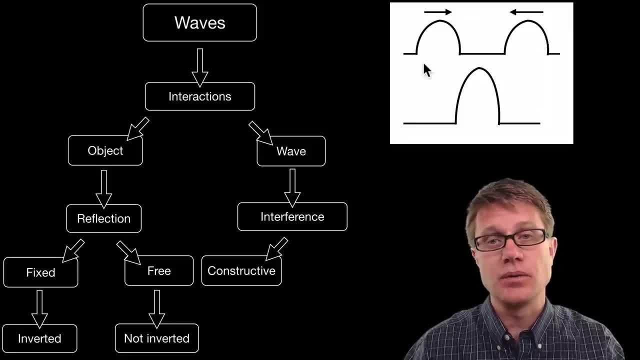 come towards each other and they are both on the top. So what do we get When they hit, we get one big wave. We are adding those waves together, So we are constructing a bigger wave. If it is destructive, we are on either side. And what do we get? We cancel each other. 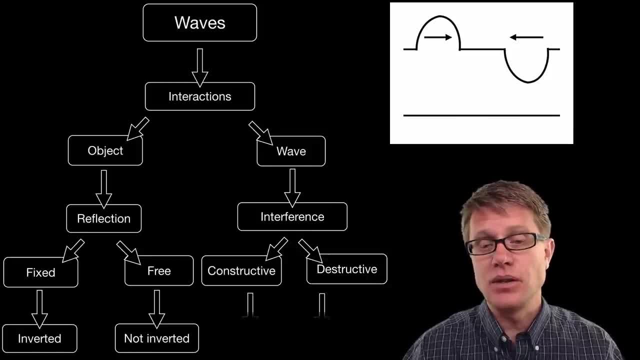 out. So we are destroying the size of that wave. We use the law of superposition to figure out how big that wave is And it is really easy If you are one centimeter on top on both of those waves and it is constructive. 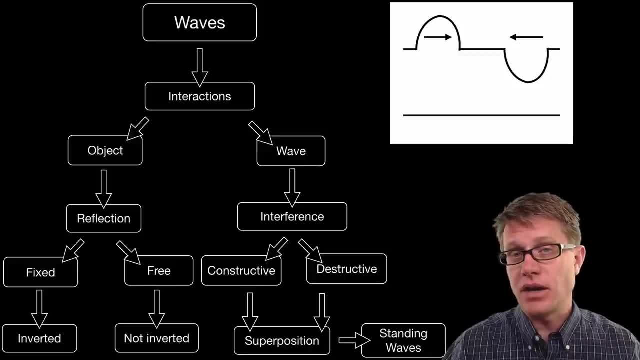 we just add 1 plus 1, and we get 2.. And so, as waves bounce back and forth, what we can do is we can build up what are called standing waves, Waves that appear to not move, but what they really are is the addition of the waves bouncing back and forth. And so let's 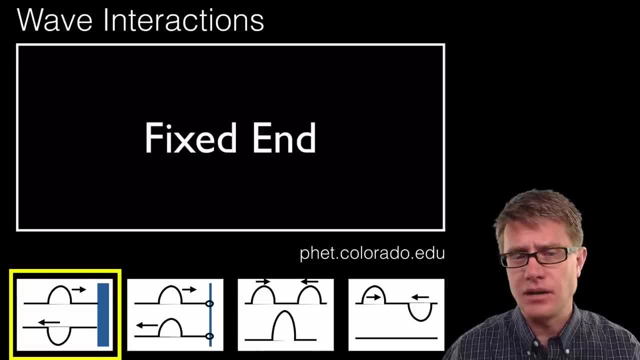 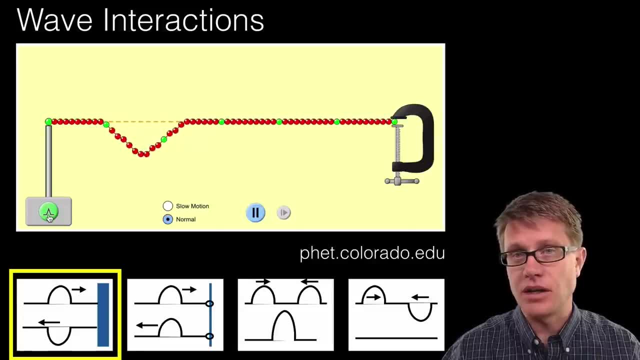 look at this using a PHET simulation. Let's start with a fixed end. So remember, if it goes into a fixed end, watch what happens. If it goes into a fixed end, what happens As it comes back. it is inverted. So it went down on the top and it came back on the bottom. 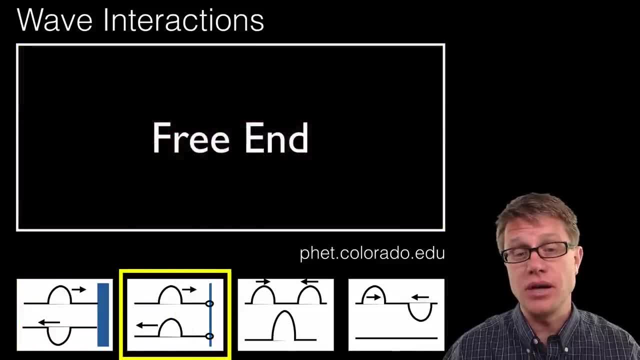 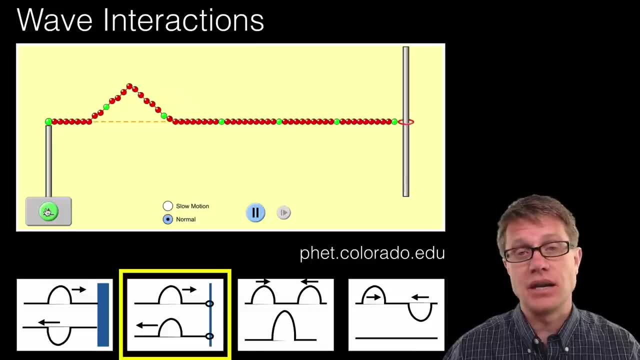 Watch what happens if we now change that from a wave interaction where we have a free end, So it has the ability to move up and down, It comes back on the same side And so, again, it depends on what we are hitting as to how we come back. But we are coming back, We are. 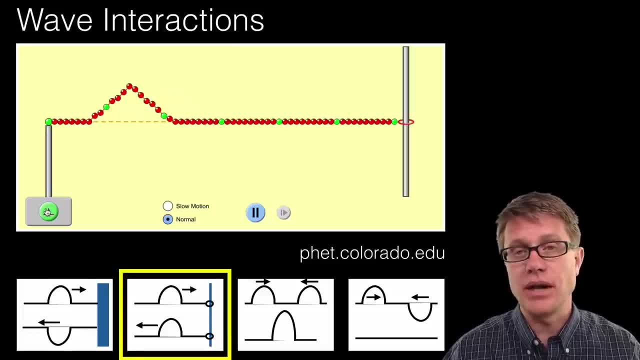 being reflected. Now let's move into interactions between waves, when waves hit waves, And so that can be, remember, constructive or constructive, And that is what we are going to do here. It can be constructive or it can be destructive, And so let's start a wave moving down. So 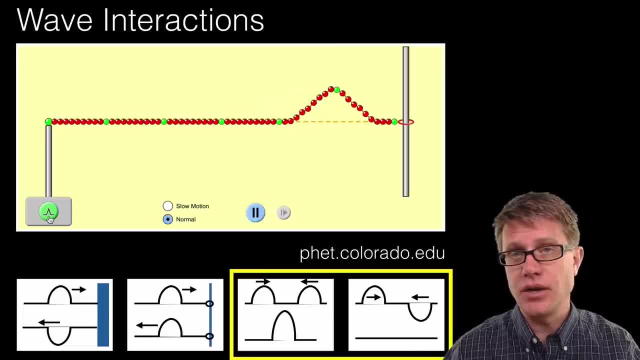 let me pause it for a second. Do you remember what is going to happen? We are hitting a free end, And so what is going to happen to that wave when it comes back? You should have said: it is on the same side And so let's do that. We were right, But you can see that. 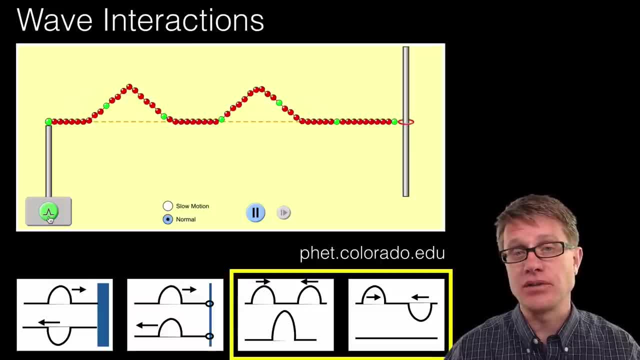 I also generated a wave that is now moving from the left. These are about to hit each other, And so what is going to happen as they interact? Well, we should see constructive interference And let's watch what happens. So we get one big wave right when the wave 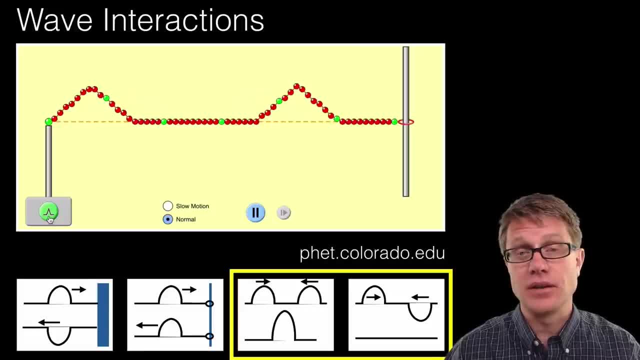 and they come together. Now what is going to happen to the wave on the left? Well, it is hitting a fixed object, So it should be inverted. And the one on the right should hit an object that is free, And so it should not be inverted. So now what is going to happen? 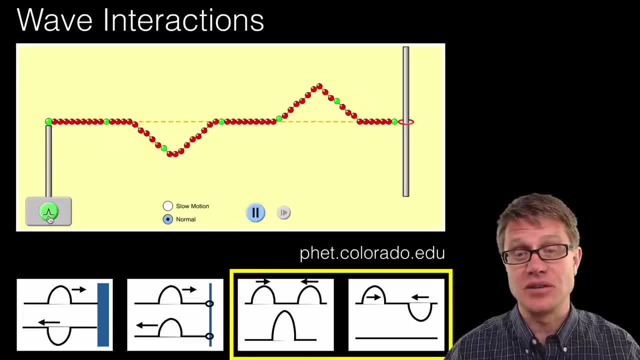 when they hit. You should have figured this out. This is destructive interference now, And so watch what happens when they hit. They should cancel each other out, And we can just see this reflection and interference and interference and reflection- again Example of this. So 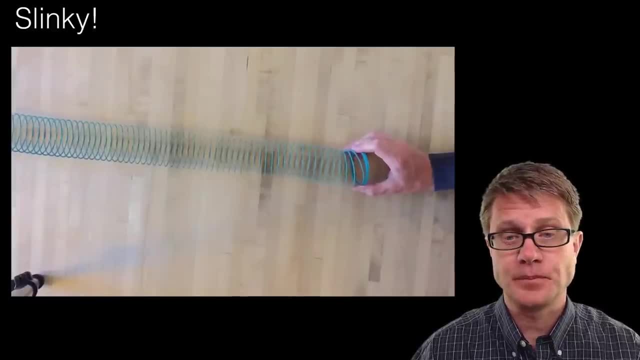 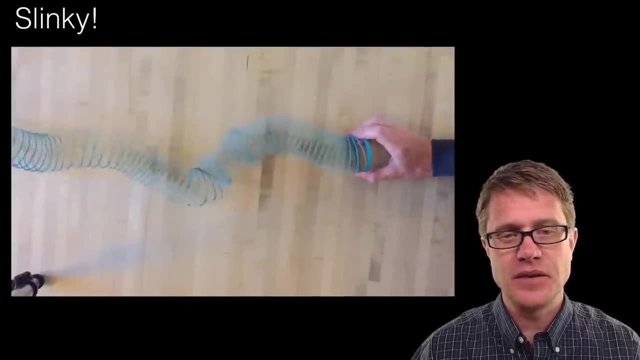 I am going to take a slinky and really send a pretty big wave. We will do this in slow motion, You can see. I kind of almost knocked my camera over. So the wave is moving to the left. It hits a fixed object and it was inverted. It hit my hand, which is a fixed object, And 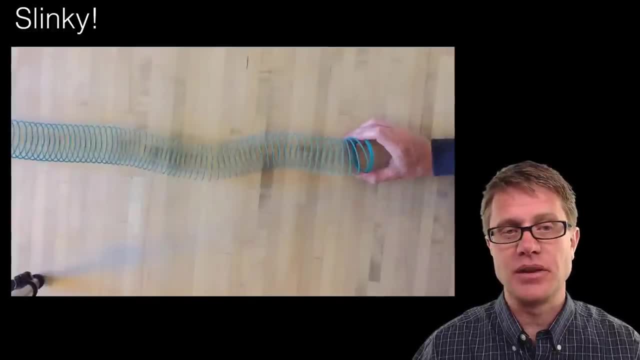 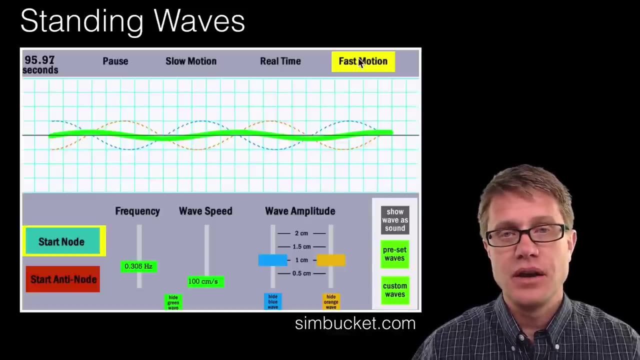 then it is going back in the other direction. So that is going to be that reflection of the wave. Now what will happen is if those waves keep bouncing back and forth, and back and forth, and back and forth, they are adding to and subtracting from each other, And so